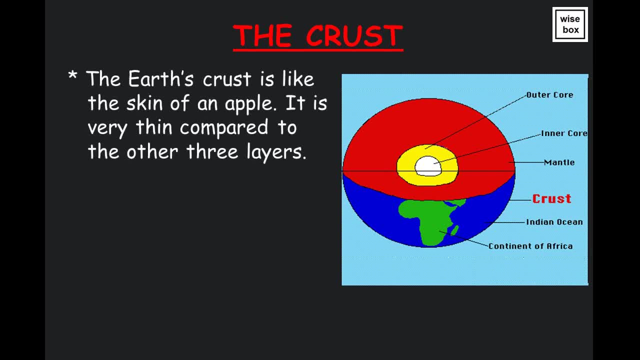 The earth's crust is like the skin of an apple. It is very thin compared to the other three layers. The crust makes up about 1% of the earth. The crust of the earth is broken into many pieces, called plates. The oceanic crust is very dense and is mostly made of basalt. 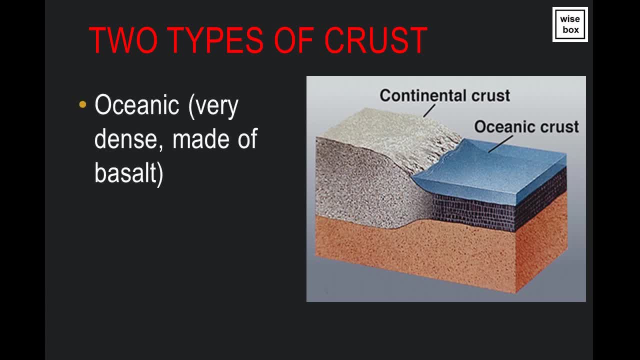 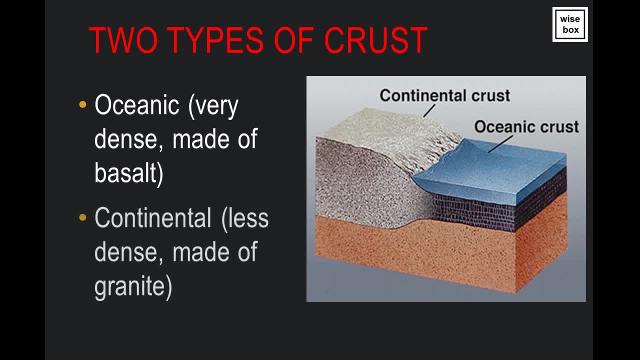 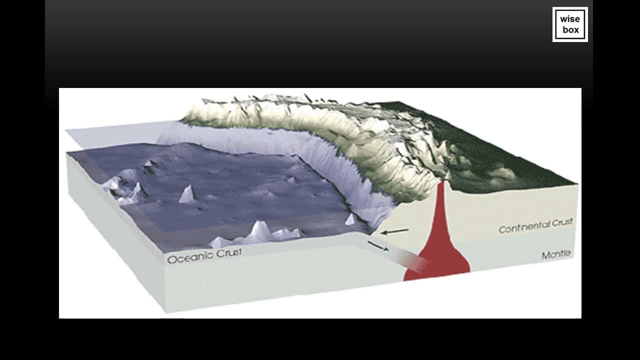 The continental crust is less dense and is mostly made of granite. The oceanic crust is very dense and is mostly made of granite. The oceanic crust is very dense and is mostly made of basalt. The oceanic crust is very dense and is mostly made of granite. 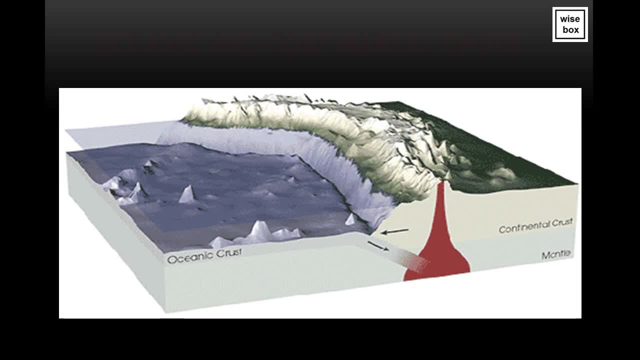 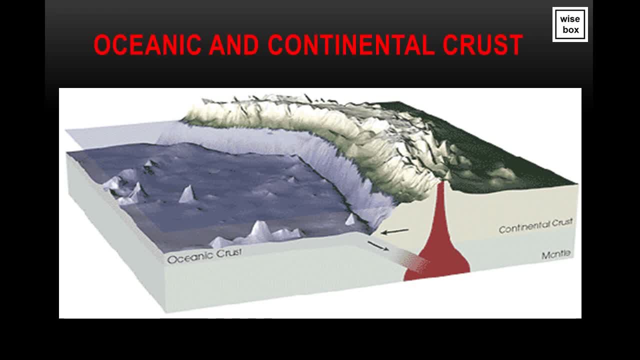 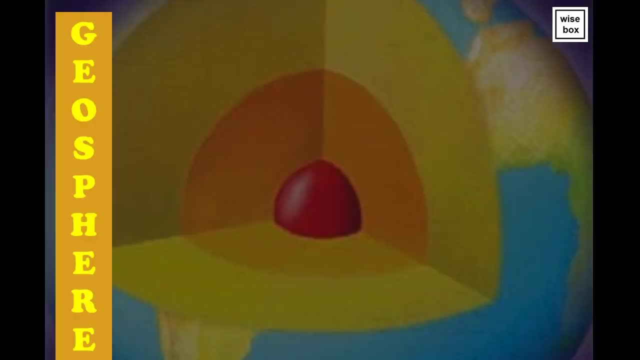 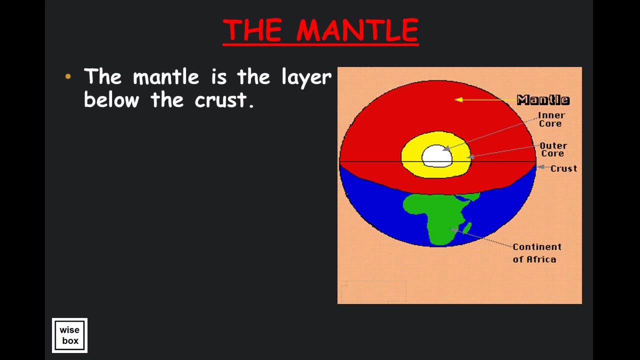 The continental crust is very dense and is mostly made of basalt. The continental crust is very dense and is mostly made of granite. The oceanic crust is very dense and is mostly made of basalt. The mantle: The mantle is the layer below the crust. 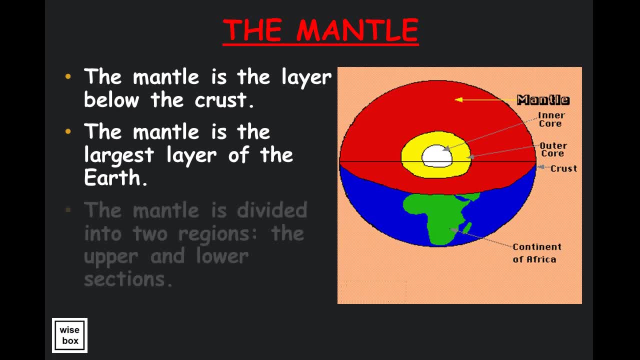 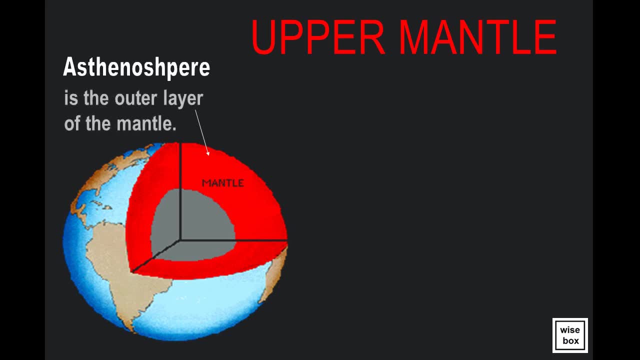 It is the largest layer of the Earth. The mantle is divided into two regions: the upper and lower sections. The asthenosphere is the outer layer of the mantle. The region just below the crust and extending all the way down to the Earth's core is called 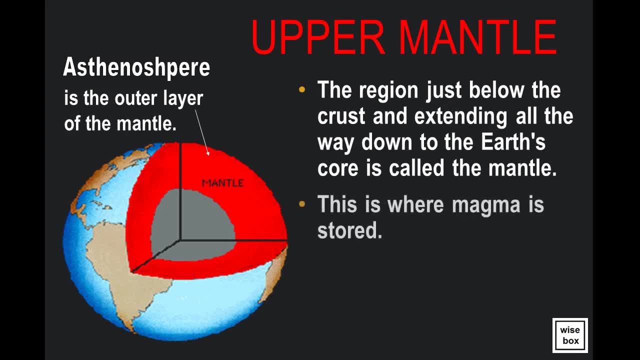 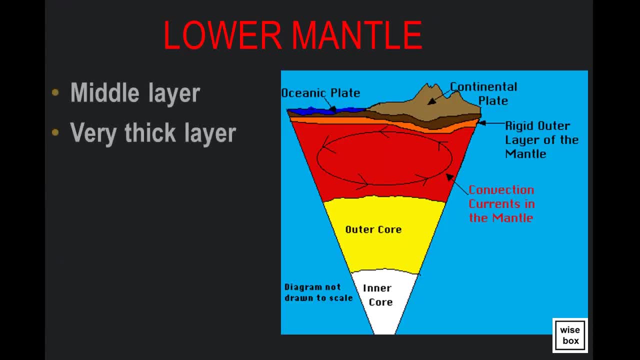 the mantle. This is where magma is stored. Molten rocks in the asthenosphere is rigid. The lower mantle is the middle layer and is very thick. Molten rocks are fluid and moving in a circular motion called the convection current. 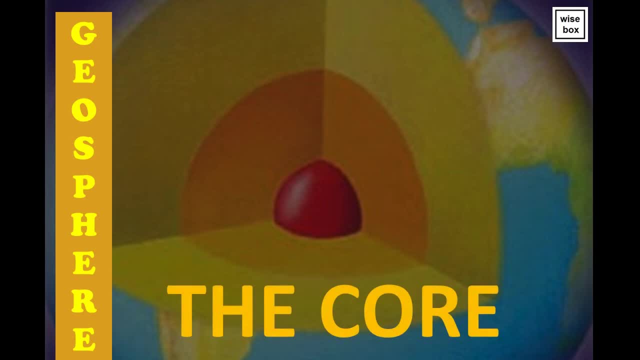 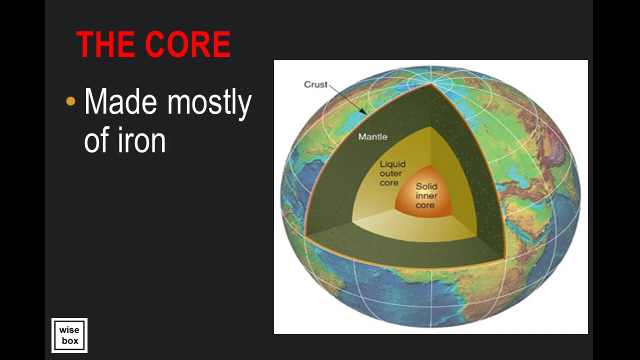 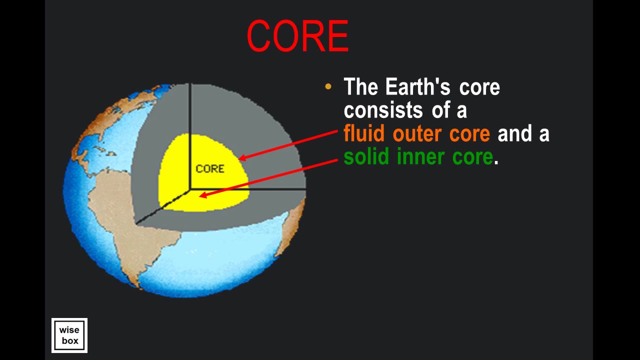 The core. The core is made mostly of iron. It is one-third of the Earth's mass and is very hot. The Earth's core consists of a fluid outer core and a solid inner core. Because the outer core contains iron, when it flows it changes its shape.